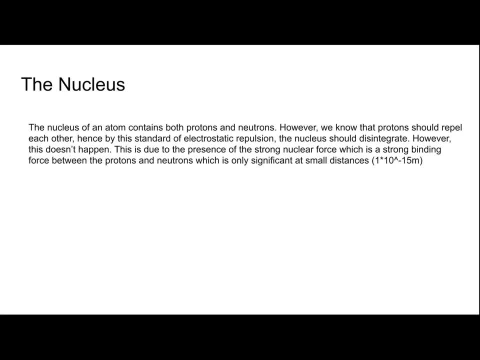 Right. so, starting off, we're going to be looking at the nucleus of an atom. So the nucleus of an atom contains? It contains both protons and neutrons. we should know about this from our chemistry. however, we know that, since, like charges repel, therefore the protons should theoretically repel each other by electrostatic repulsion force. 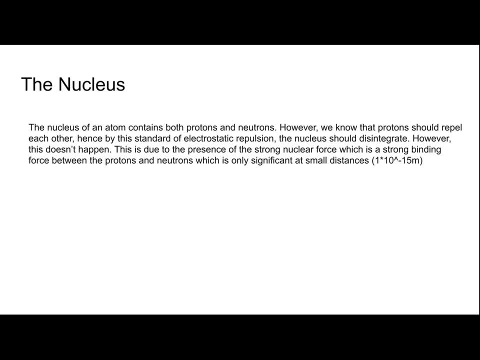 So therefore, according to this, that the nucleus should disintegrate, so the protons should repel each other, so that all of the protons will be separated from each other and the nucleus will disintegrate. However, this actually doesn't happen, because we have our nucleus is tight. 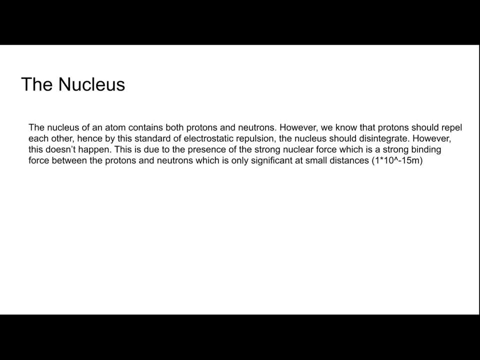 Very. The nucleus and the protons and neutrons are very tightly bound together so obviously they're not being repelled. So this is due to the presence of the strong nuclear force, which is a strong binding force between the protons and neutrons. 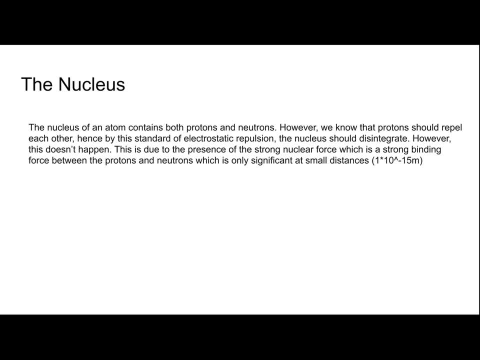 So there is a very strong binding force between the protons and neutrons. however, this binding force is very significant at very small distances. So at very small distances, this force will overcome the electrostatic repulsion. therefore, the nucleus will be held together. 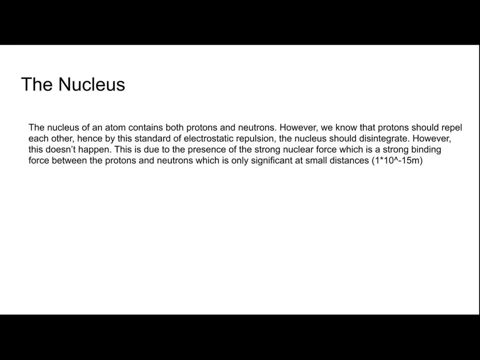 Because the nuclear binding force bigger than the electrostatic repulsion. However, this is only significant at very small distances. so bracket here we have. it's only about approximation is 1 times 10 to the power, negative 15 metres. 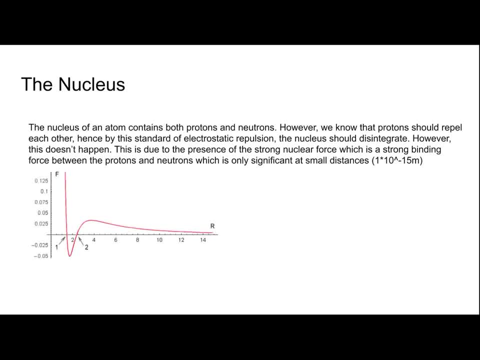 so that's very, very, very small distances there. Alright, so here's a graph of the strong nuclear force with distance, As you can see, when it's above the x-axis it's actually a repulsion force, but with the small distances where it's below the x-axis, that is, when it's. 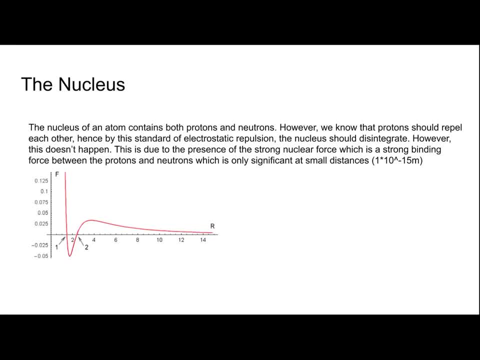 a traction force. Okay, So it's a very strong attraction force that can overcome the electrostatic repulsion, Alright. so a side note: so in a nucleus, where are the protons and neutrons, the? therefore, we refer to the protons and neutrons as a. 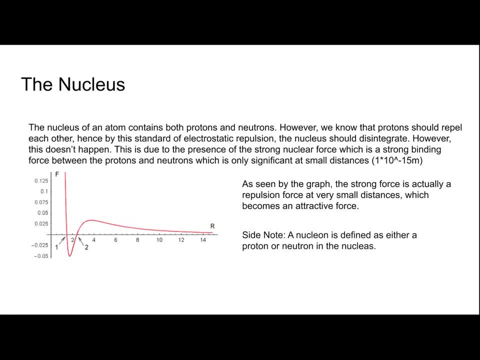 nucleon. so a nucleons can either be a proton or a neutron. So a newtron is 2 protons, which basically has aономin in it. so since neutron is nuclear, nucleon is a proton or a neutron inside the nucleus, So the nucleus can undergo nucleus. 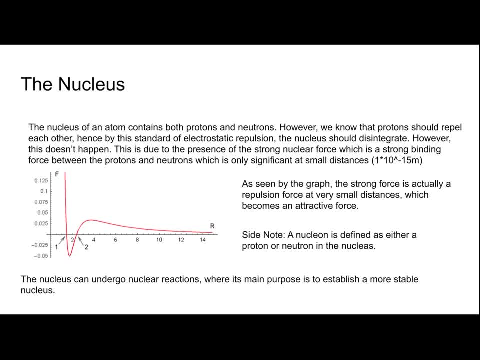 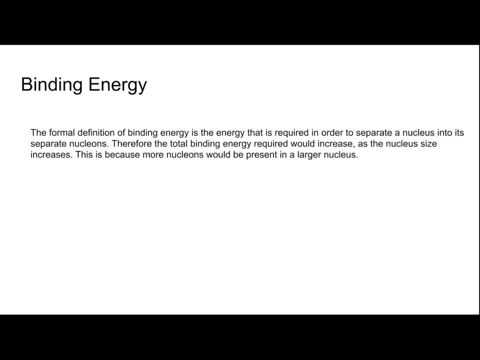 reactions and the main purpose of the nuclear reactions. the main purpose is to establish more stable nucleus. Alright, so what is the binding energy? The formal definition of the binding energy is the energy that is required in order to separate a nucleus into a separate nucleon. 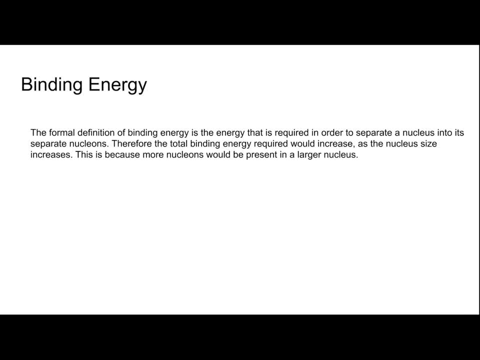 So if I have a nucleus that is very tightly bound together, me as a person, I have to do work- or not necessarily me, but something has to do work on this nucleus in order to separate these into its separate nucleons. So, separate the protons into sorry, separate the protons and 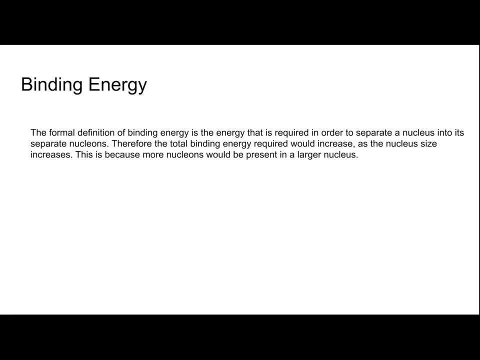 the neutrons into, so separate them individually. So once we separate each of them individually, the total amount of work done that is equal to the binding energy of the nucleus. So therefore the total binding energy would increase as the nucleus size increases. 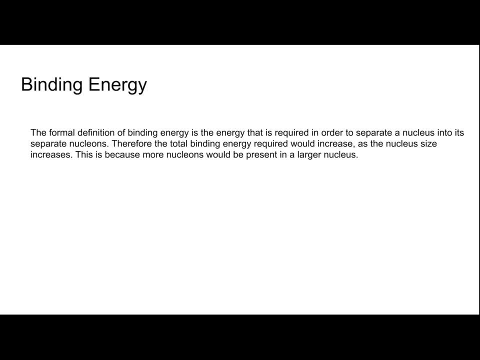 because there's going to be more and more protons and neutrons and therefore it will require more work, more binding energy, in order to split these protons and neutrons into their individual. into their individual protons and neutrons, Alright. so, likewise, the binding energy can also be defined as the energy released when 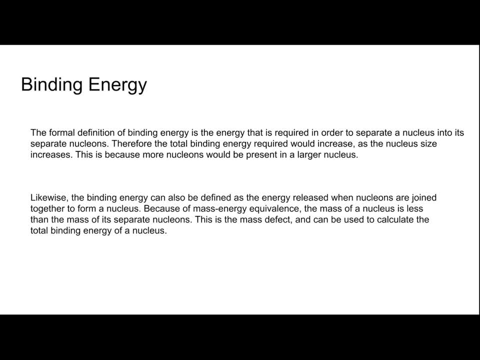 nucleons are joined together to form a nucleus. So when nucleons are joined together, so when I have my protons and my neutrons, I'm going to join them together- the strong nuclear force is going to bind them tightly together and some 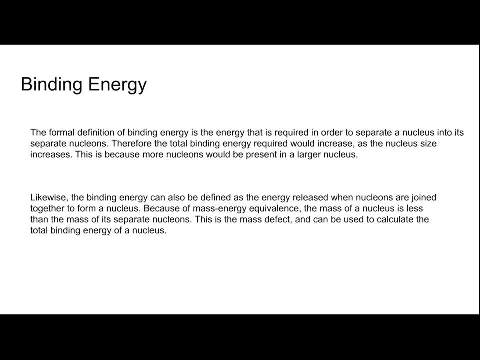 some of these energy is going to be released. Because of the mass energy equivalence theory, the mass of the nucleus is actually going to be less than the mass of its separate nucleons, So the so the separate the mass of the separate nucleons. 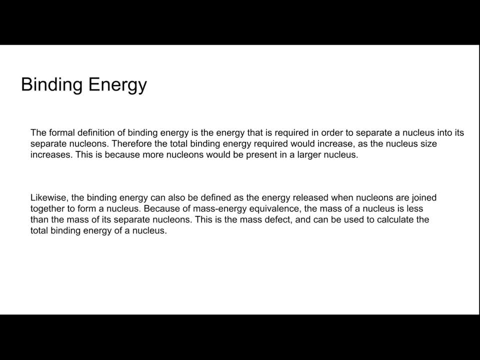 that's the protons and the neutrons individually, will actually be larger than the mass of the final nucleus, because once the näu- sorry, once the protons and neutrons bind together, some of that energy is lost. um, some of that energía is released or another. 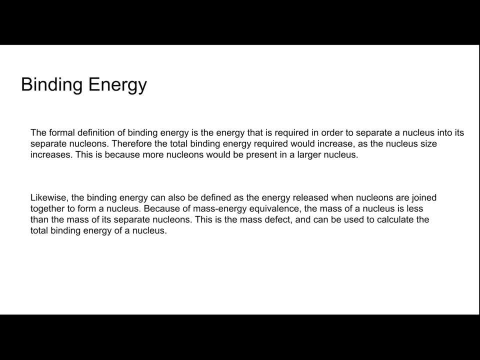 another word for that- is liberated. Some of the energy is liberated. therefore, the final, final mass of the nucleus is actually less than the mass of the individual protons and neutrons. This is called the mass defect, the mass defect of a nucleus, and this can. 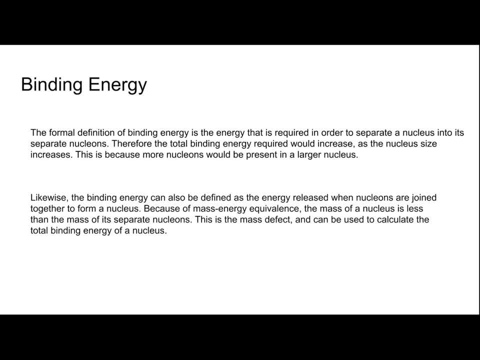 be used to calculate the total binding energy of a nucleus, And that is your Einstein's formula, that is, the E equals to mc squared. That can be used to find the binding energy of a nucleus. However, that doesn't necessarily mean that large nuclei are more stable. It. 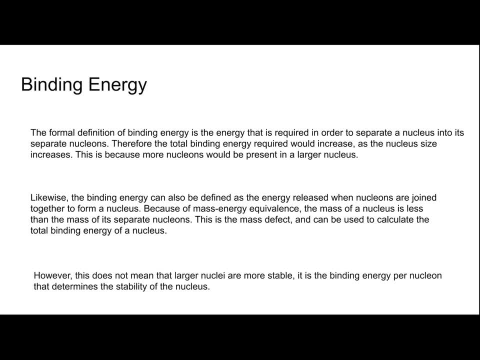 is the binding energy per nucleon. so the amount of binding energy per nucleon, so the amount of work I need to do to separate the nucleus into its individual protons and neutrons. So per nucleon it actually depends on the stability of the nucleus. And likewise when 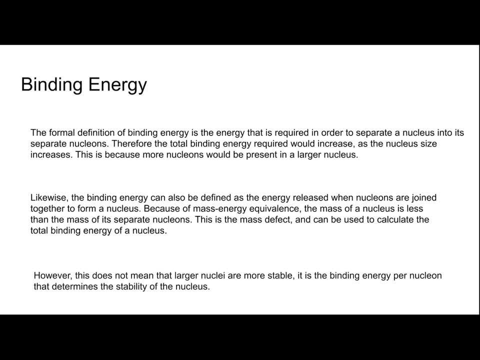 I do work to separate the nucleus into its separate nucleons. the work I do, the energy I do, the work is actually transferred into the system. Therefore, the mass of the separate nucleons will also will actually be bigger than the mass of the nucleus. So that's another. 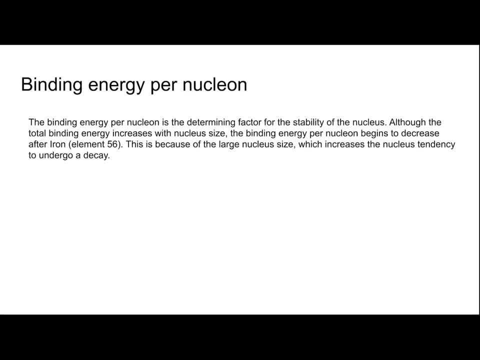 way to explain it: Binding energy per nucleon. So the binding energy per nucleon is the determining factor of the stability of the nucleus, Although the binding energy increases with nuclear size. like I said, more nucleons, therefore, more work needs to be done. The binding energy: 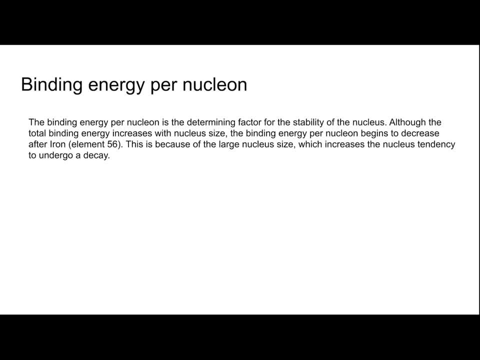 per nucleon actually begins to decrease after iron. element 56.. So sorry, it's actually meant to say element 26 on the periodic table. My mistake there. Okay, so nucleon begins to decrease after iron. So after iron, as the nucleus gets bigger. 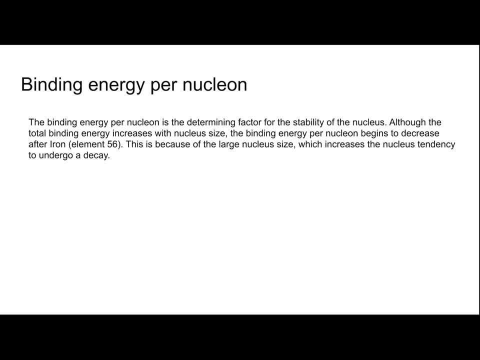 the binding energy actually increases because there's more nucleons, However, the binding energy per nucleon per nucleon begins to decrease. So therefore the stability actually begins to trend downwards. So because when there's a large nuclear size, this actually 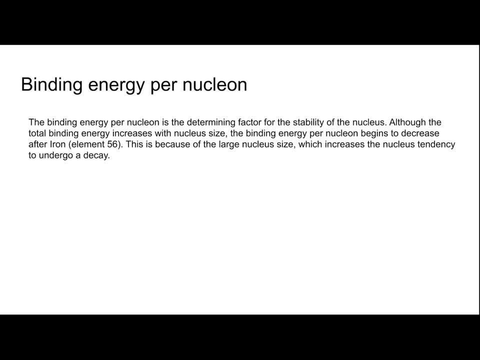 increases the tendency of the nucleus to underbind. That means하면there'sh gol a decay. so that could be a beta decay, alpha decay and gamma decayнали- advent radiation. We'll talk about that in part two. so here we have a graph of 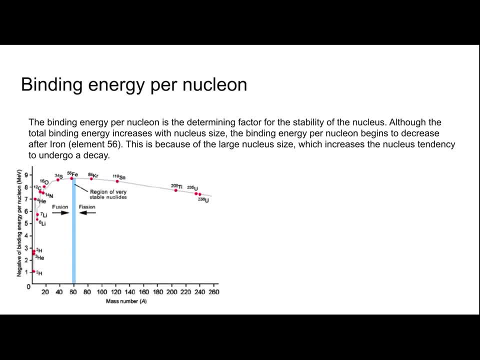 the binding energy per nucleon- This is the y-axis- is a mega electron volts. One mega electron alto is equal to fone point times in the power of negative thirteen joules. So as we can see here, very small nuclei are very unstable, as well as the bigger nuclei. 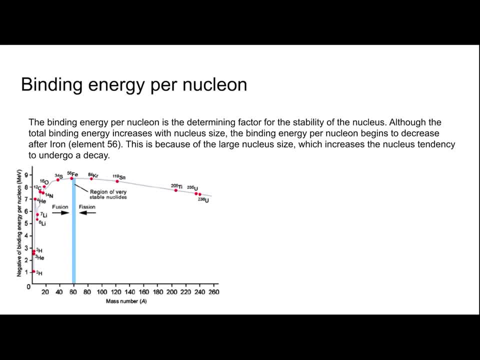 the stability begins to decrease, As we can see here. the peak of this graph is that our iron. So iron actually has the largest binding energy per nucleon. therefore, it is considered the most stable nuclei, So, as seen in the graph, the BEPN. so that's just an abbreviation. 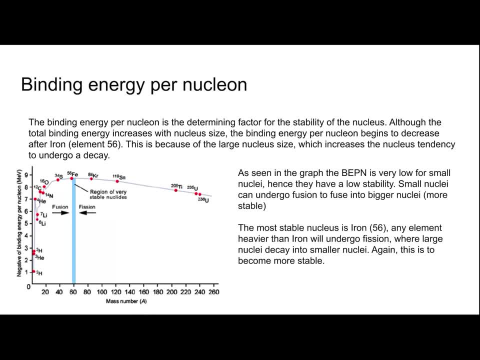 for binding energy per nucleon. it's very small for small nuclei. they have low stability. The most stable nucleus is iron-56.. Sorry, iron is actually element 26 on the periodic table. but any element heavier than iron will undergo fission. 56 is the mass number of 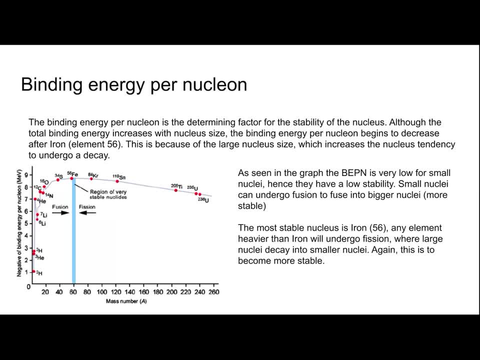 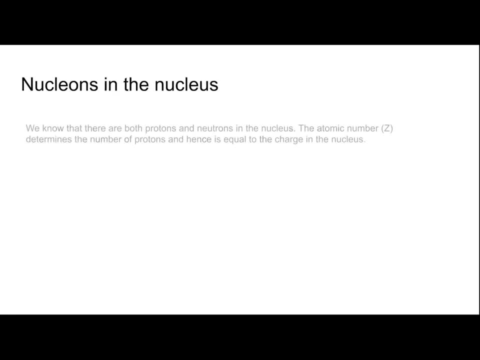 iron. the atomic number of iron- that's the position on the parallel table- is actually 26.. So any element heavier than iron will undergo fission, where large nuclei decay into smaller nuclei again to become more stable. So nucleons and the nucleus. so we know that. 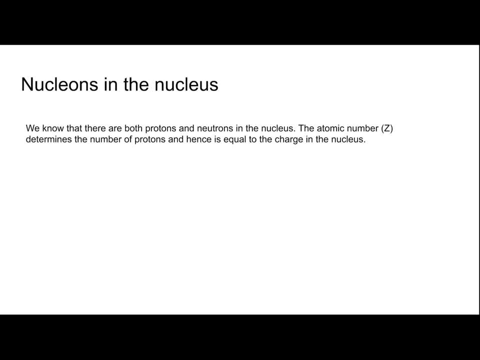 there are both protons and neutrons in the nucleus, The atomic number that's sometimes abbreviated as Z. that determines the number of protons, and hence it is equal to the charge in the nucleus, because we know that the charge of the neutrons is zero. but 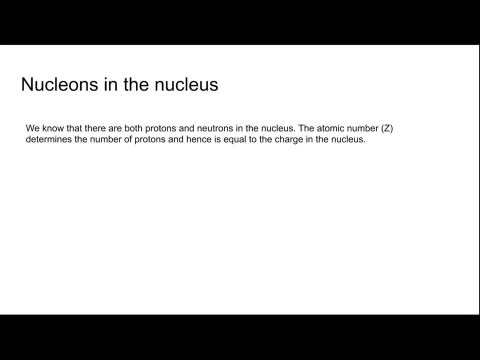 the charge of the protons is positive one. Therefore, the number of protons is equal to the charge on the nucleus. The mass number is also known as the nuclear number, so mass number, nuclear number. However, it is the amount of nucleons in the nucleus, so that's. 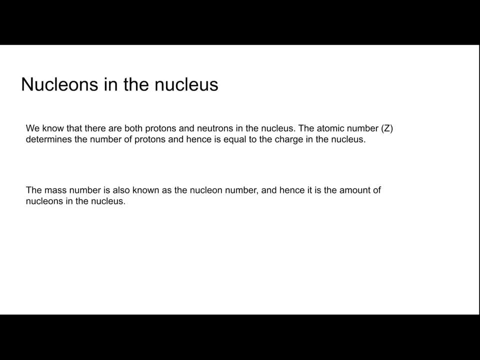 the amount of protons plus the number of neutrons in the nucleus To represent elements in the nuclear equation, the following model is present: So we have X. X is representing our element, so it's an abbreviation. Therefore, if we said iron, iron would actually be Fe. 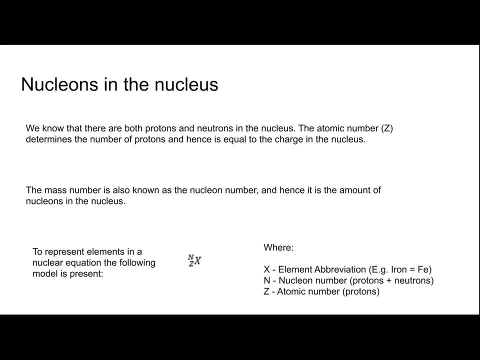 that's its abbreviation. Therefore X in this case would be Fe. N is the nuclear number, so that's the number of protons plus the neutrons, so that's also the mass number. Z is the atomic number, and that's the number of protons in the element. 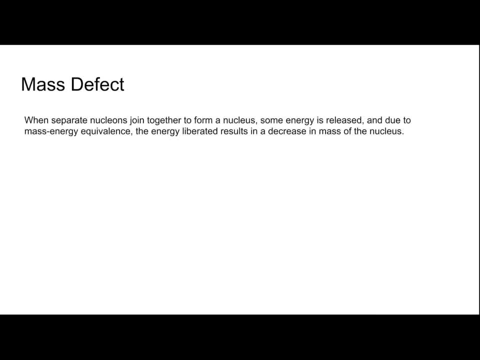 Alright. mass defect: So when separate nucleons run together to form a nucleus, some energy is released and, due to mass energy equivalence, the energy liberated results in a decrease in mass of the nucleus and this is known as the mass defect. This can actually be used. 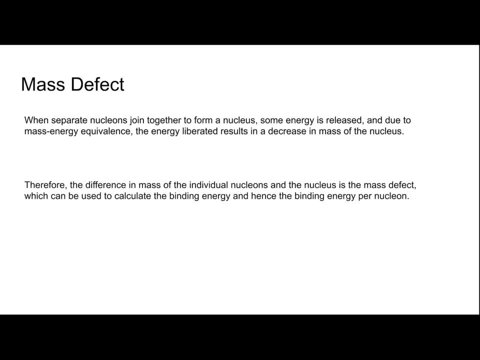 to calculate the binding energy, and hence the binding energy per nucleon of a specific element. So Einstein's famous formula- E equals to MC squared- can help us find the binding energy from the mass defect or vice versa. Here's a quick example. So calculate the binding energy per nucleon of an iron: 56 atoms. 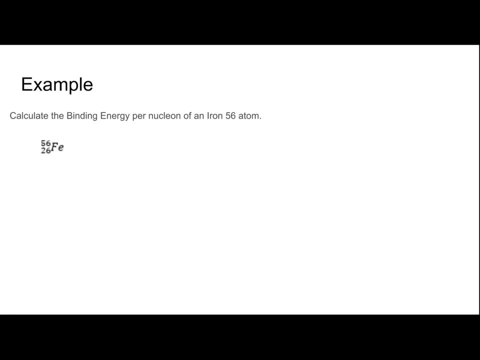 so 56 is the mass number. So here is the, here is the, here is iron we have. mass number is 56, atomic number is 26, and here is the data we need, So our mass of a proton. I told 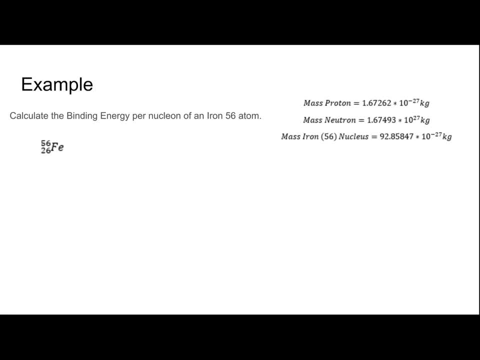 you is 1.67262 times the power of negative 27 kilograms. Mass of the neutron is equal to 1.67262.. 1.67493 times 10 to the power of, that should say negative 27 kilograms, so 1.67493 times. 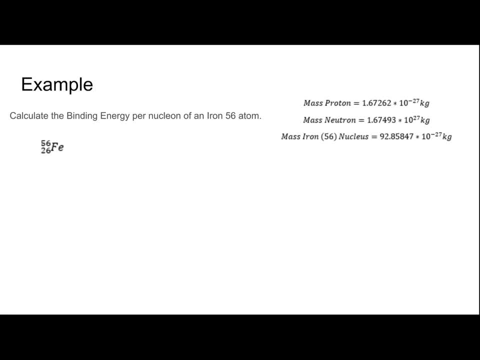 10 to the power of negative 27 kilograms, and mass of the iron nucleus is 92.85847 times 10 to the power of negative 27 kilograms. Alright, so when we're doing this nuclear reaction standard, it's very important that. 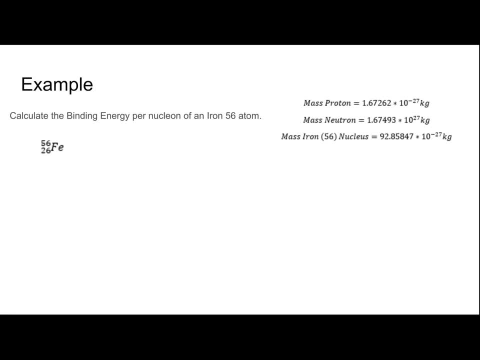 all our decimal places are being grounded consistently at a very large amount of decimal places. So, as we can see here, mass of proton over starter is given to 5 decimal places. so your final answer should theoretically also be in the 5 decimal places. 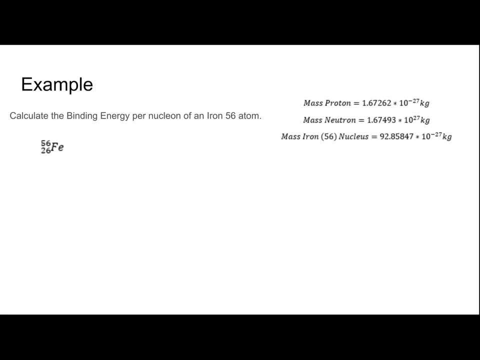 So to give a go at this question, calculate the binding energy per nucleon of an iron 56 atoms. So pause the video, give this question a go and when you're done, keep watching the video to find out the answer. 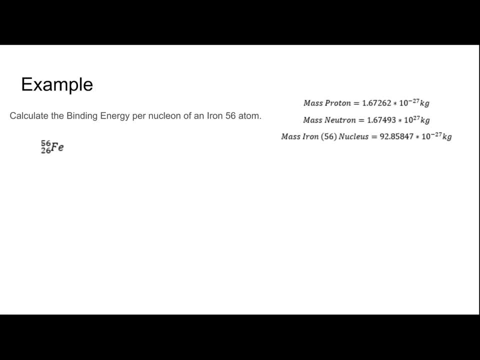 Alright, so how do we start this question? So we know that the mass defect is similar to the difference in mass between the nucleons and the mass of the nucleons. So we know that there's actually 26 protons in iron. we know that because the atomic number 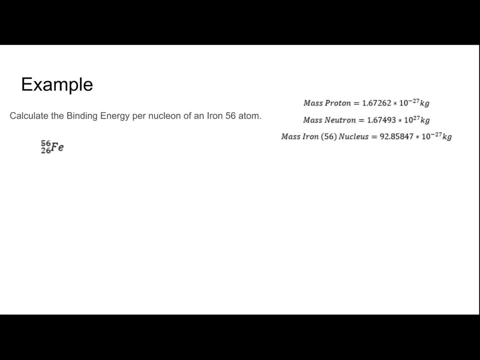 is given to us as 26.. 26 is the atomic number. that's equal to the number of protons. Therefore, we also know that the number of neutrons is actually equal to 30. There are 30 neutrons in the Fe nucleus. 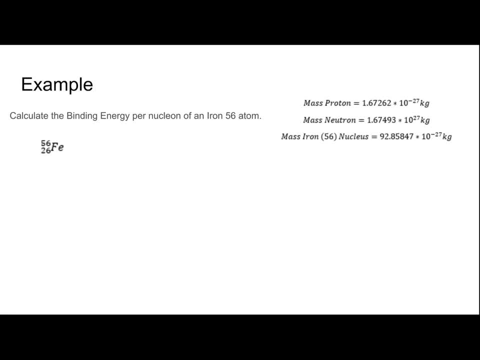 This is because the mass number is 56, and therefore because there's 26 protons. 56 minus 26. will give us our 30 neutrons. so therefore we're going to add the masses of our individual nucleons. that's our first step. so mass of nucleons we have as m, i'm going to say it's mass of nucleons mn. 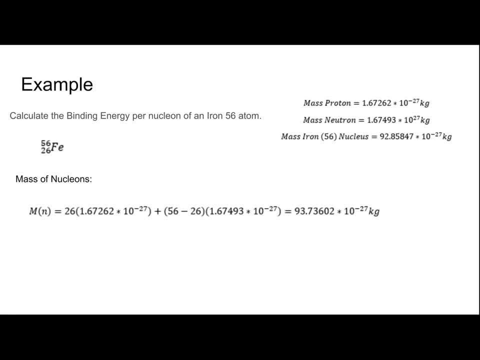 that's equal to 26 times the mass of the proton, plus 56 minus 26, which is 30- 30 times the mass of a neutron. that should give us the final mass is 93.73602 times 10 to power off negative 27. 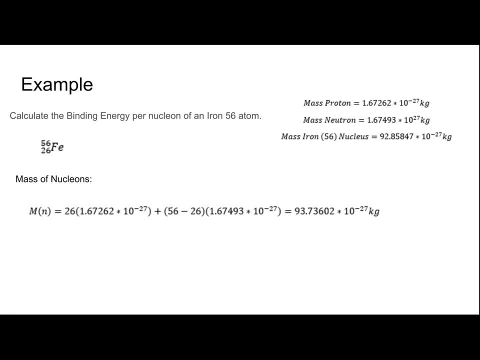 kilograms. now we're going to find the difference between the mass of the nucleons and the mass of the iron nucleus. so therefore, the mass defect we know is actually equal to the difference in the mass, which is actually 8.77550 times 10 to the power of negative 28 kilograms. 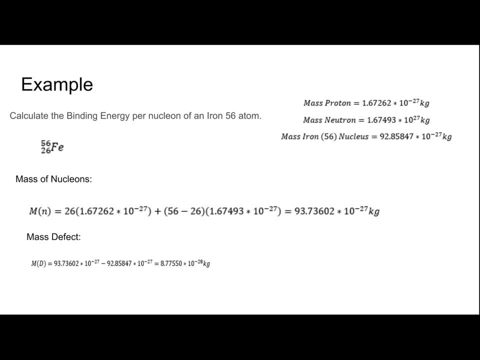 so now we're going to have find the total binding energy for the iron 56 atom. to find the total binding energy we need to use einstein's formula. that's e equals to mv squared. okay, that's right. what am i saying? so that's equal to that equal. that's equal to e. equals to mc squared. okay. 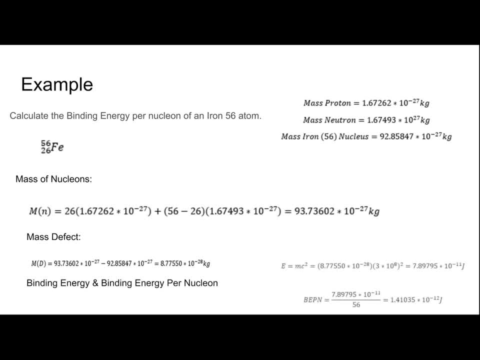 so we're going to say that binding energy energy and binding energy per nucleon. so we're going to say our binding energy is E equals to MC squared. that's going to give us the answer of 7.89795 times the power of. 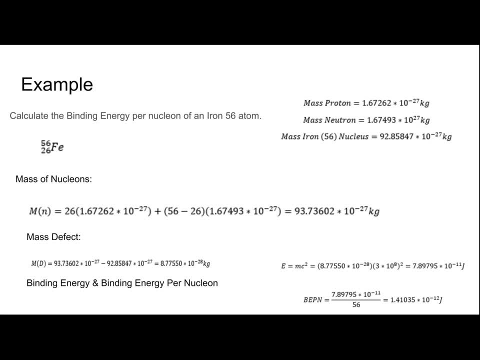 negative 11 joules. That's the total amount of binding energy for the iron 56 atom. However, the question is asking us to find the binding energy per nucleon. So the binding energy per nucleon is simply will be the total binding energy divided by the total number of nucleons. 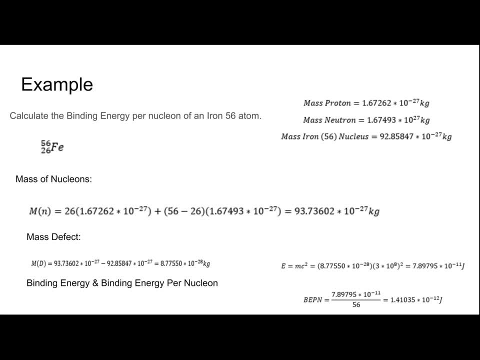 in the atom. In this case we have 56 nucleons. therefore, our binding energy per nucleon is our total binding energy divided by 56, and that should give us our final answer of 1.41035 times 10 to the power of negative 12 joules, And that's our final answer. 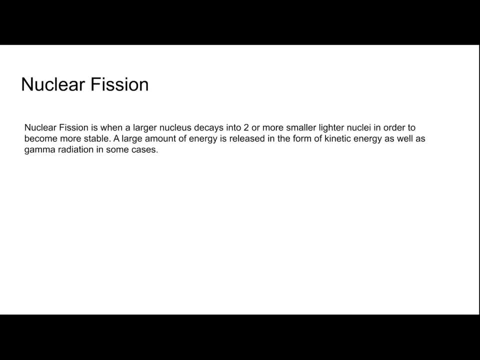 Alright, so nuclear fission. So nuclear fission is when a larger nucleus decays into two or more smaller, lighter nuclei in order to become more stable. So that's a key word. Bigger nuclei: we saw in the previous video. So that's a key word. Bigger nuclei: we saw in the previous video. 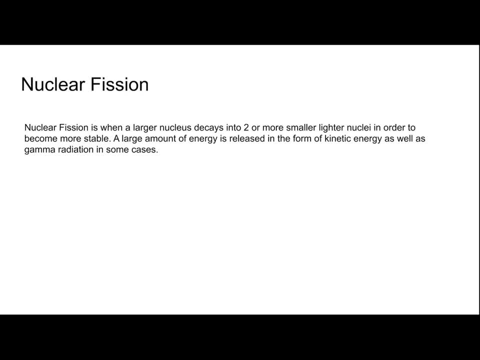 In the graph above. after iron 56 nucleus, the stability began to decrease. So we see these very big, very big, sorry, we see these very big nuclei. So we know that, because they are very big, we know that the strong nuclear force, the strong nuclear force I was talking in slide two. 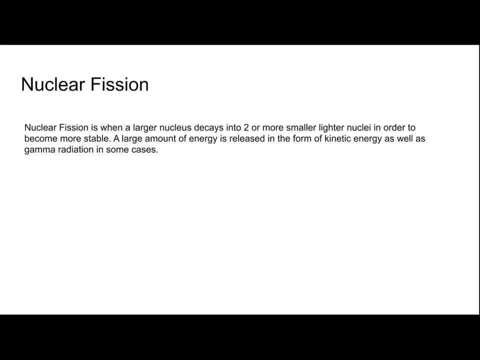 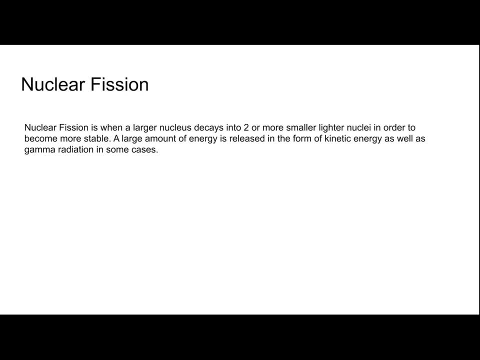